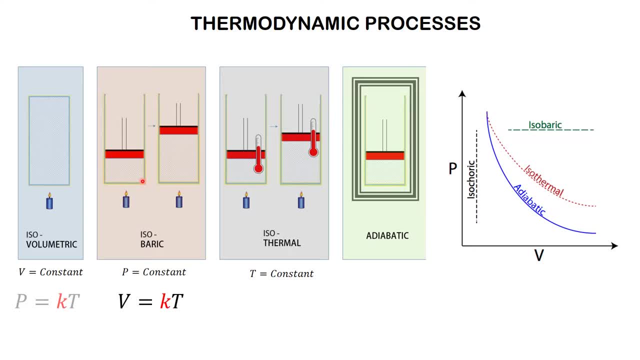 pressure is applied. When the container is heated, the gas expands and the temperature of the gas increases. The pressure is also increased. Here the ideal gas equation can be written as: V is equal to kT, because pressure is constant. The P-V diagram for this process is again straight. 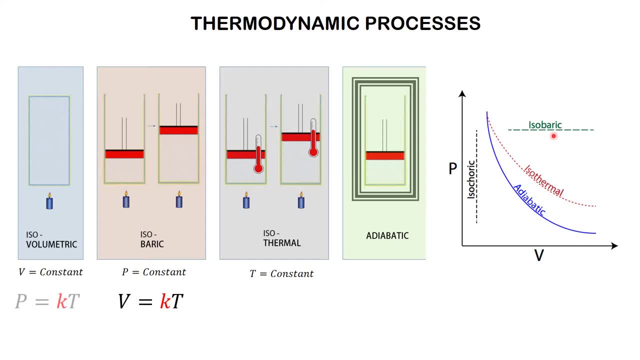 forward because pressure is constant. It's a line which is parallel to the volume axis. In an isothermal process, one end of the container has a movable piston, So the pressure is also increased. When the gas is heated, the volume in the container can change The conditions. 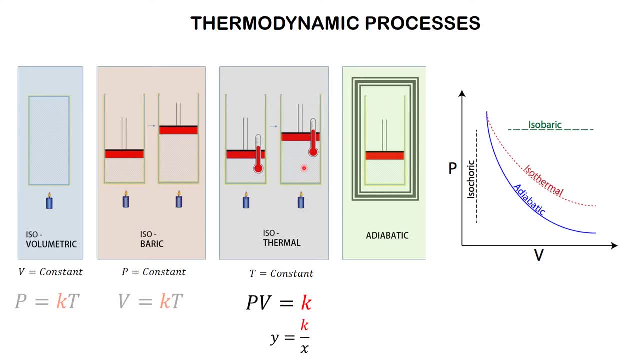 are maintained such that both pressure and volume can change, but the temperature in the container remains constant. So our ideal gas equation can be written as: PV is equal to k, which is a constant, because N, R and T- all three are constant When we plot P versus. 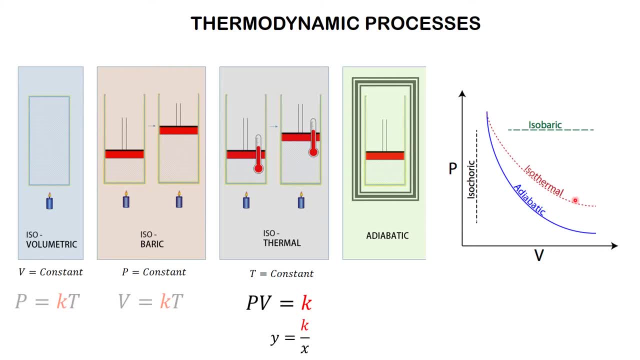 V on the PV diagram We get a downward sloping curve because this equation is like: y is equal to 1 by x. So for different values of k or for different values of temperature we get different downward sloping curves. also notice that on the isobaric curve the volume here and the temperature. 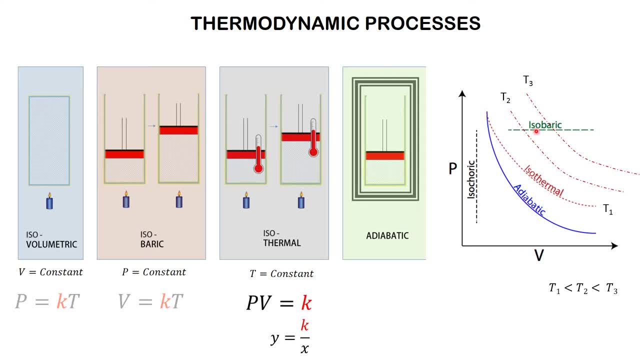 here versus volume here and the temperature here, which means that as the volume increases, the temperature increases. That means in the isobaric curve the volume here increases and increases. Similarly, where the isotherms cut the isochoric curve, we will find that 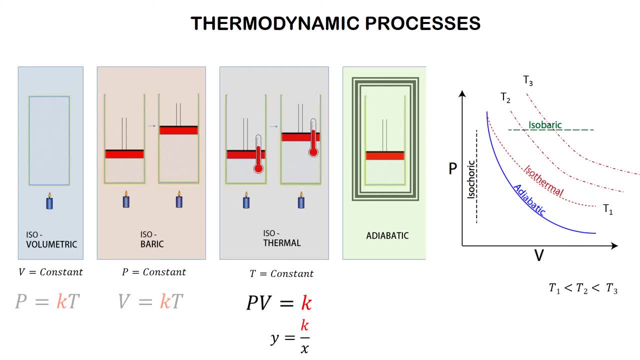 pressure and temperature are directly related In an adiabatic process. PV raised to power, gamma is a constant, where gamma is Cp by Cv, the specific heats at constant pressure and constant volume. So the adiabatic curve here is steeper than the isothermal curve because 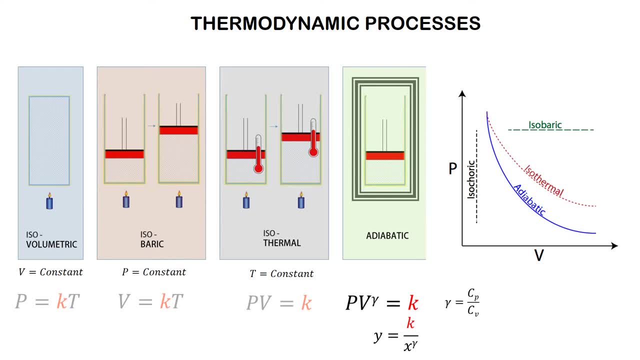 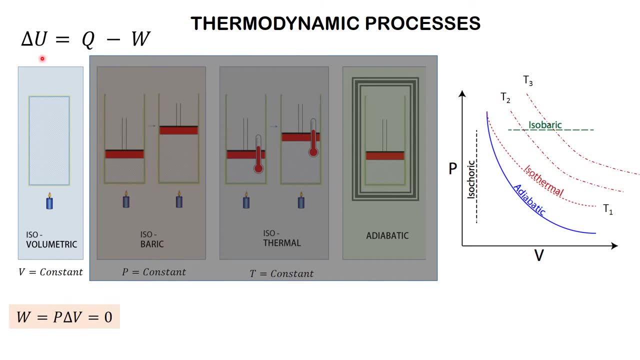 of this constant gamma, which is the exponent of V. As per first law of thermodynamics, the increase in internal energy of the gas, delta U is equal to the heat supplied to the gas, minus the work done by the gas. In an isovolumetric process, the work done by the gas is zero, since there is no increase.